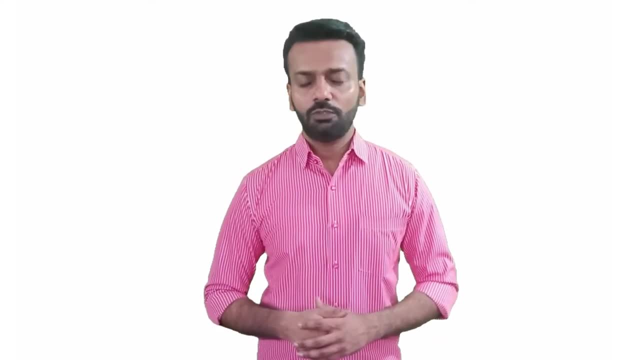 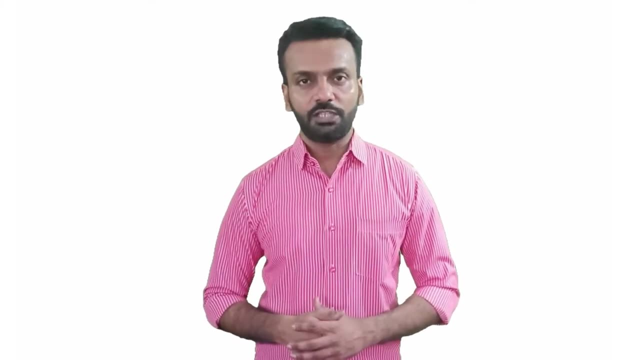 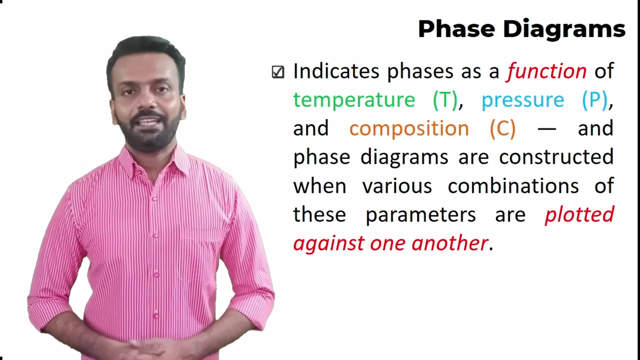 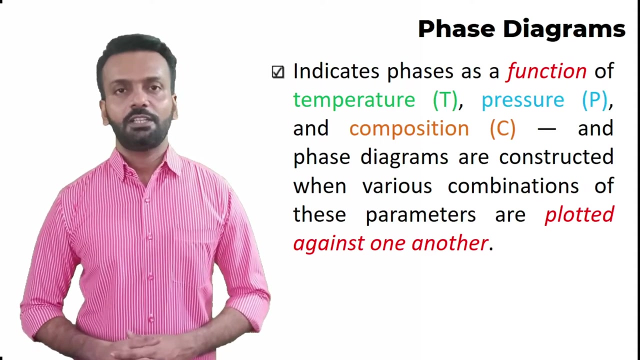 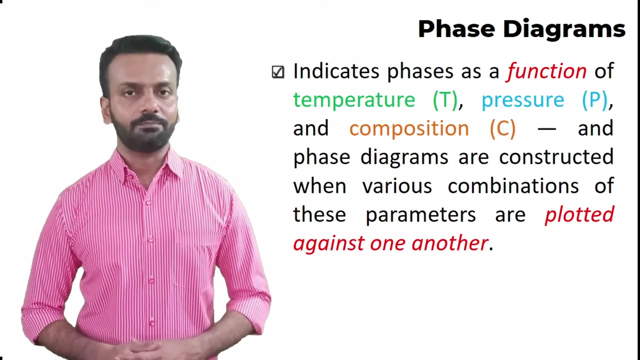 Hello friends, I am Dr Vasim Sheikh. In this video we will discuss about what are the different types of phase diagram and which phase diagram is the most important for us to study. So let us start. Let us do a recap on phase diagram. Phase diagram are nothing, but it shows phases as a function of temperature, pressure and composition, And all these different parameters are plotted against each other on the phase diagram. 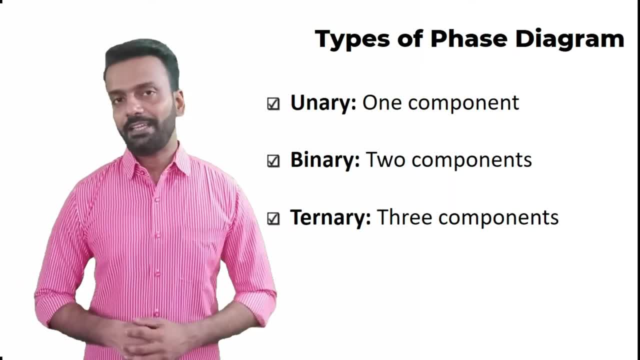 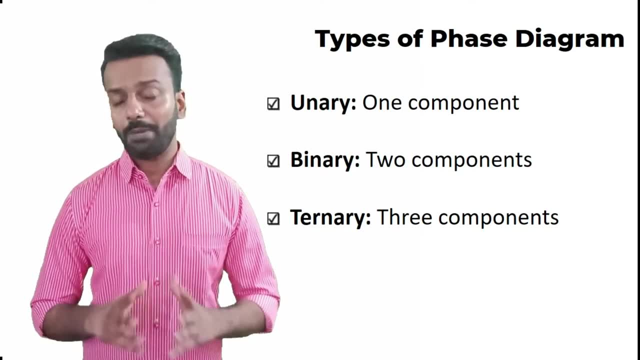 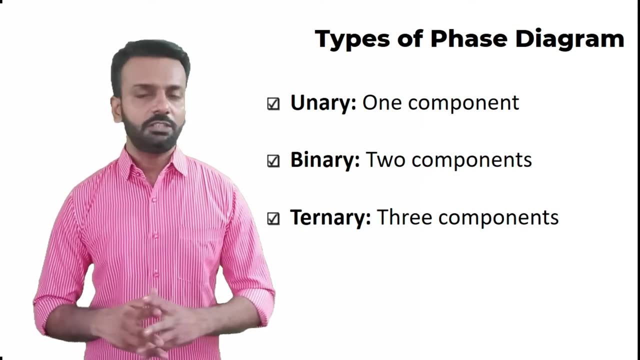 So first of all, let us list what are the different types of phase diagram. So the three types of phase diagram are: unary phase diagram, which is a one component phase diagram, Binary phase diagram, which is a two component phase diagram, And the last one is the ternary phase diagram, which is a three component phase diagram. 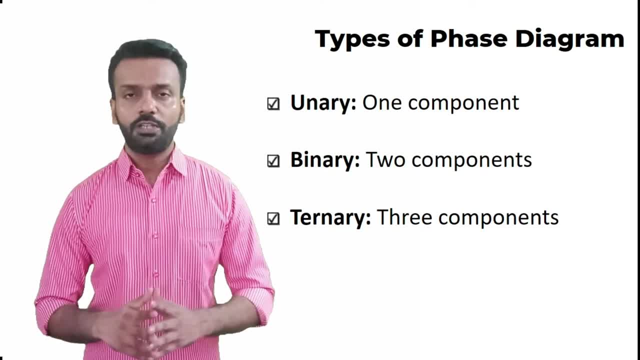 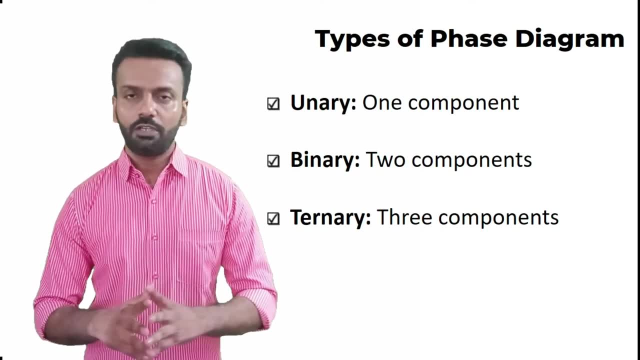 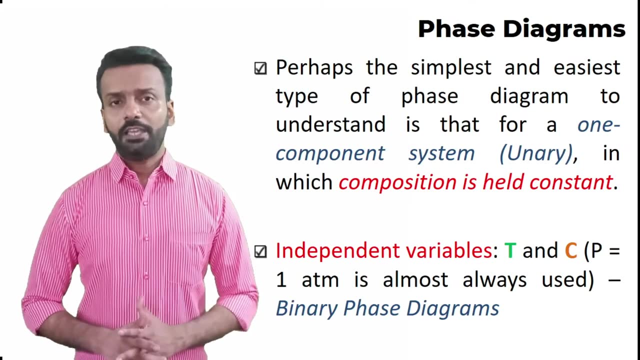 So in an earlier video we have discussed about what are the components, what are the phases and some different definitions related to phase diagram. You can refer to that video if you are not aware of the components In the phase diagram. the simplest one is the unary phase diagram, where the composition is held constant and the pressure is constant. 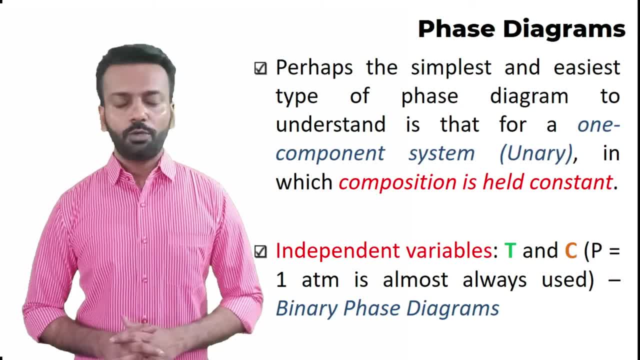 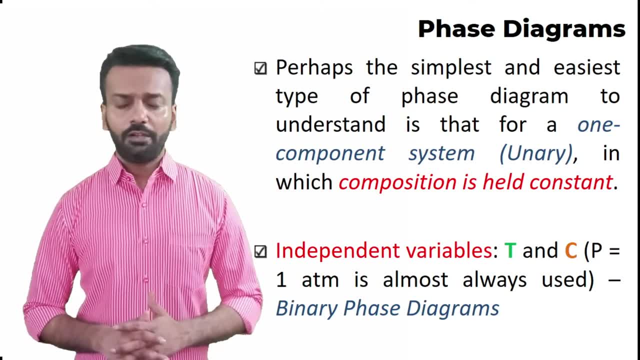 The temperature and temperature is varied. And we have one more important phase diagram, which is called as a binary phase diagram. Here the pressure is held constant and the temperature and composition is varied against each other. And this is the most important phase diagram. 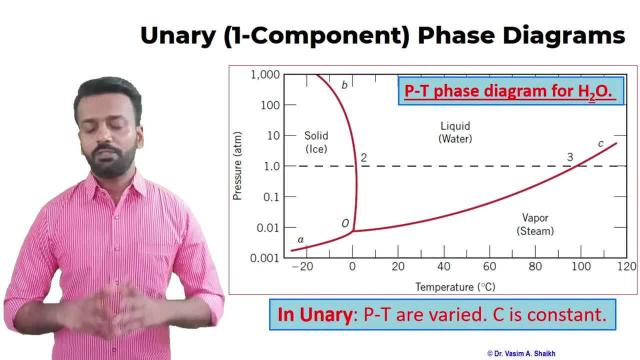 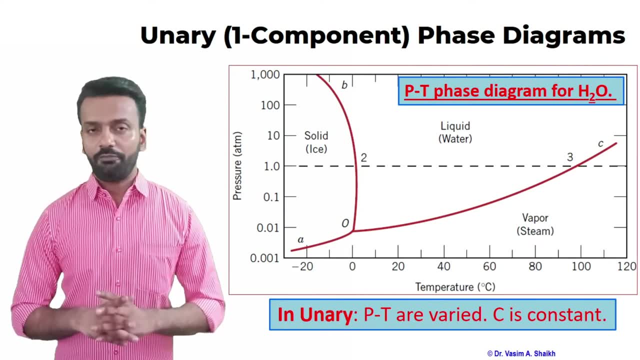 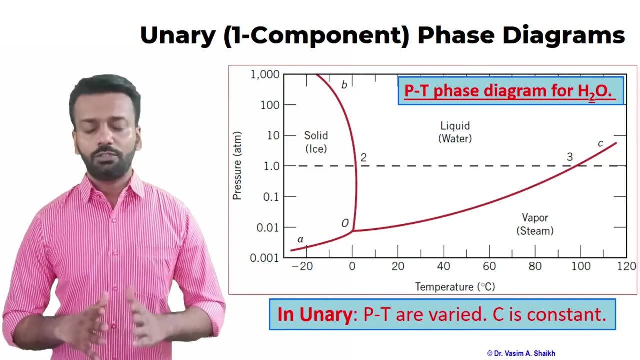 Let us take an example of unary phase diagram Here. in this image you can see that this is a phase diagram of water. Here the pressure and temperature are varied and the composition is held constant. You can see the different temperatures which are there on the x-axis and on the y-axis you have the pressure, which is varied. 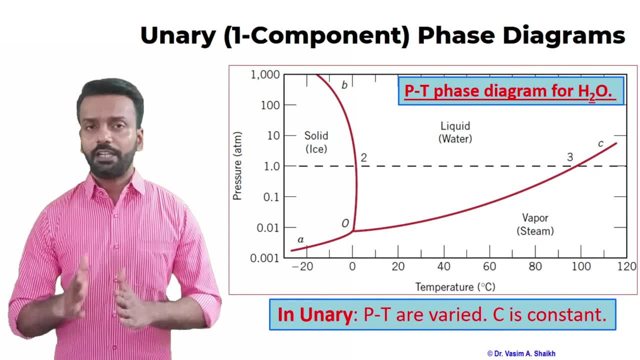 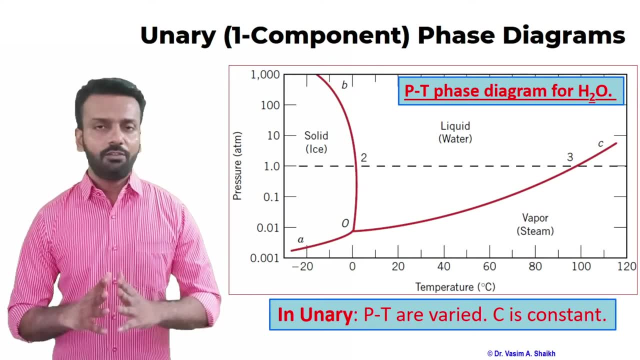 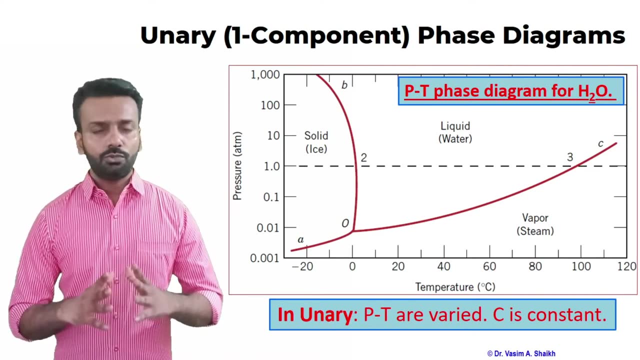 So as you keep on increasing the temperature, you can see that at one point the liquid phase will turn into vapor phase. And as you go on decreasing the temperature, at one point you can see that the freezing point will come into picture and the liquid will turn into solid. 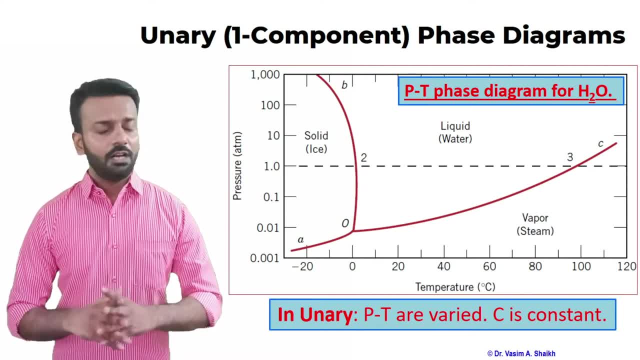 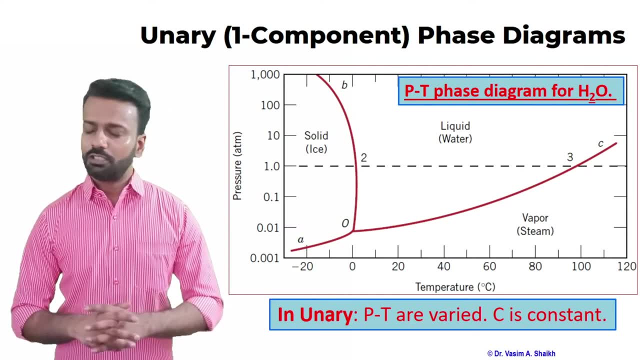 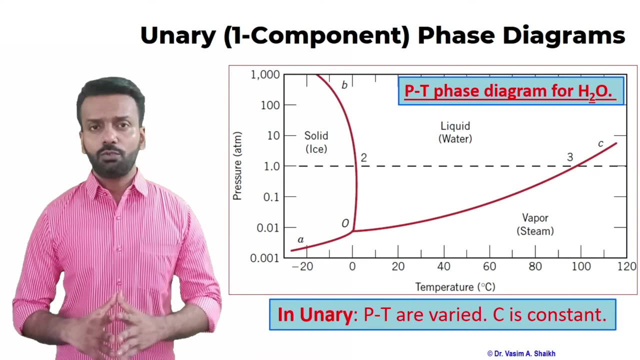 And you can read the phase diagram. So all the three phases are listed here. In this phase diagram of water, you have the solid phase, you have the liquid phase and you have the vapor or the gaseous phase. This is a one-component phase diagram because the component here is water, which is H2O, and it is a single component. 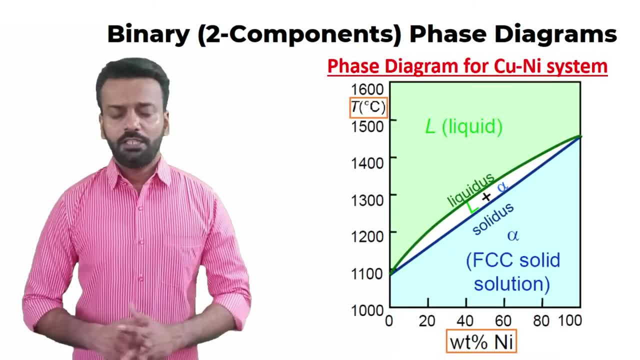 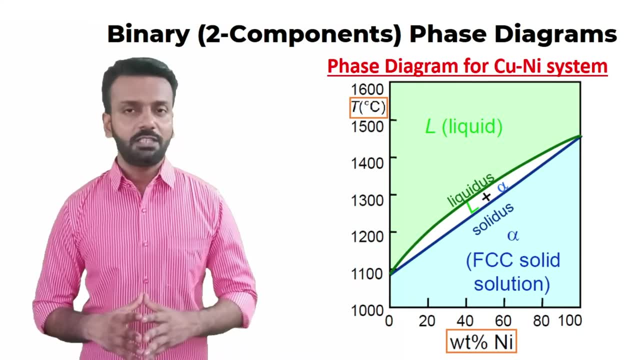 So that is why we are saying that this is a unary phase diagram. The next phase diagram is the binary phase diagram. This is the most important phase diagram as far as examinations are concerned. In most of the examination, two-component phase diagram is used. 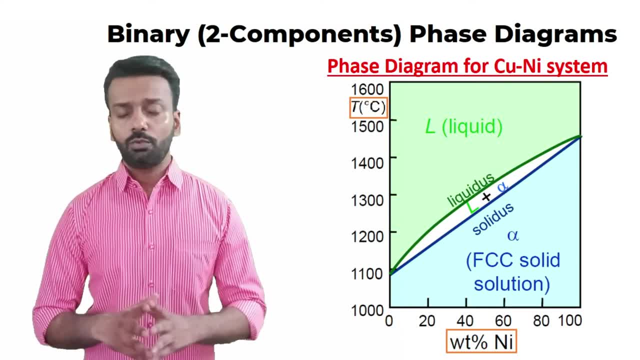 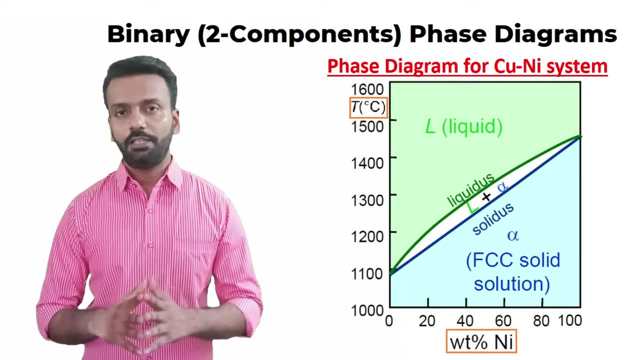 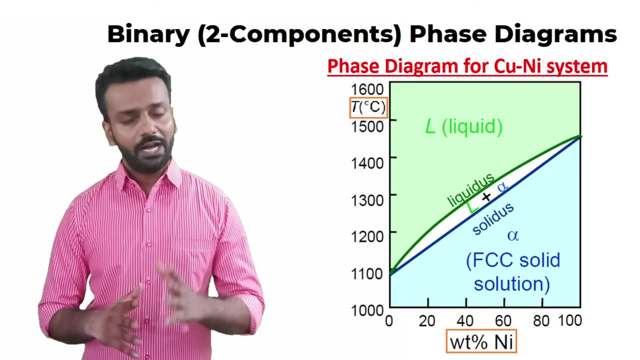 And this is a typical example of a two-component binary phase diagram. Here we can see that this phase diagram is of copper and nickel. Here, on the x-axis you can see that it has weight percent of nickel and on the y-axis it has temperature. 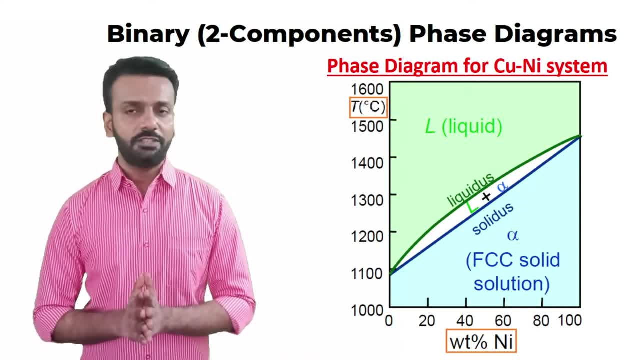 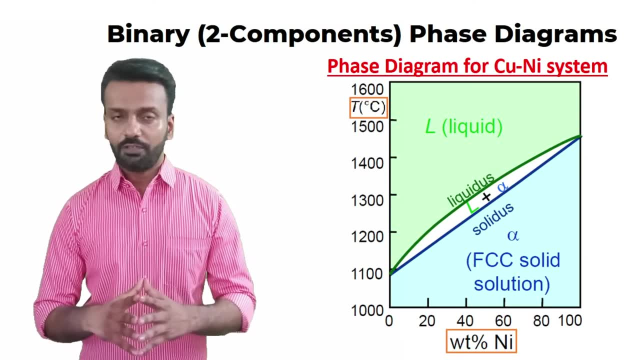 So you can see different phases which are existent. on this phase diagram. You can see a liquid phase, also denoted by L. You can see a solid phase, which is also called liquid phase. This is also called as an alpha phase. 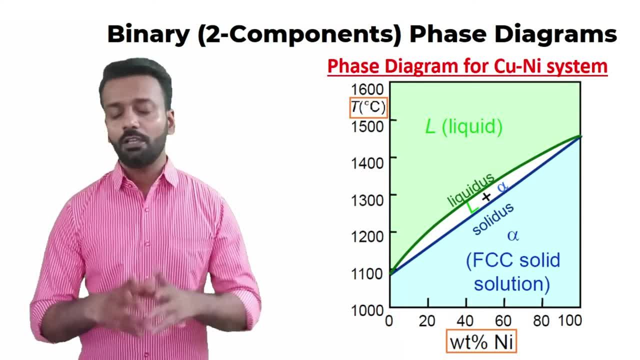 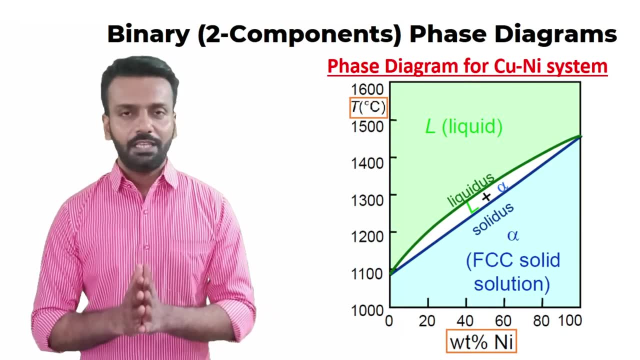 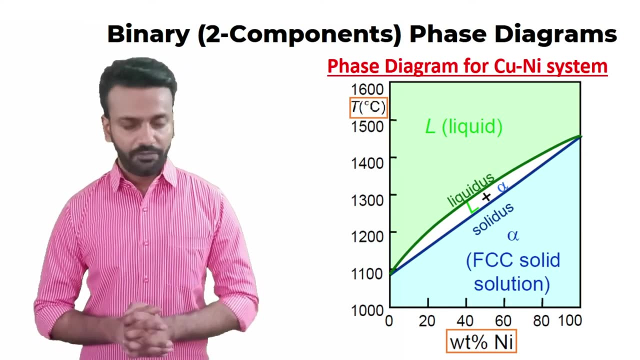 And you can see a liquid and alpha phase which is a phase field. So at this particular field or phase field, liquid and alpha- that means solid and liquid. both are existent together. So in a typical examination question you will be asked: what are the different phases that are existent on the phase diagram? 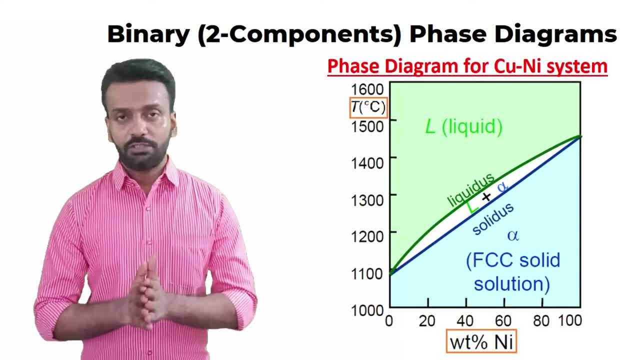 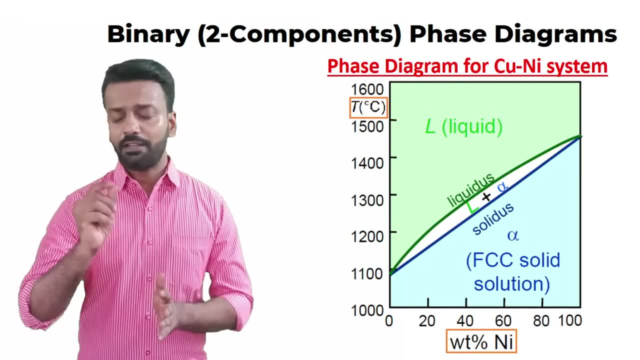 You will be asked: what are the composition of the phases? And the last question that you will be asked is: what are the different proportion of the phases Or the percentage of phases on the phase diagram at a particular point? So these are the most important questions which are related to the phase diagram. 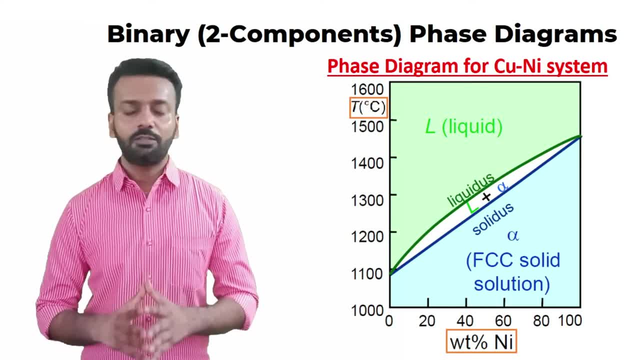 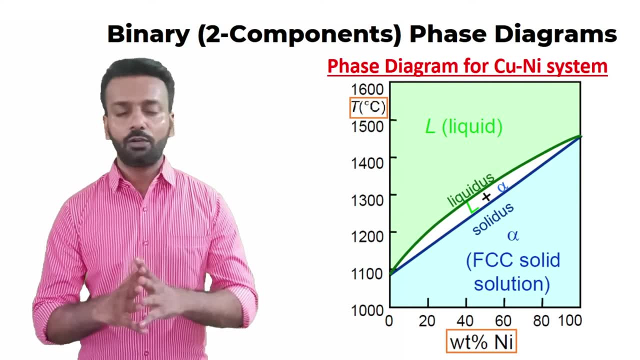 And in the upcoming videos I will be discussing about how to find out what are the phases, what are the phase composition and what are the different proportion of phases, which we can find out on a phase diagram. The next one is the ternary phase diagram. 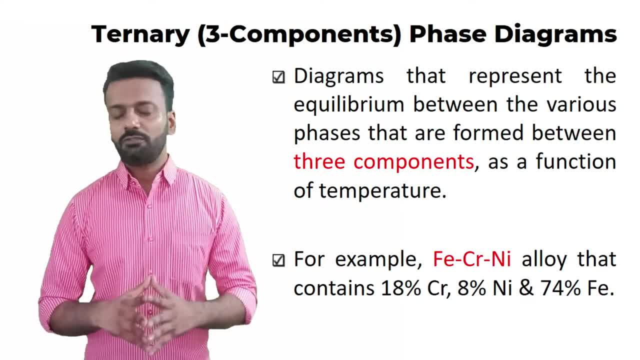 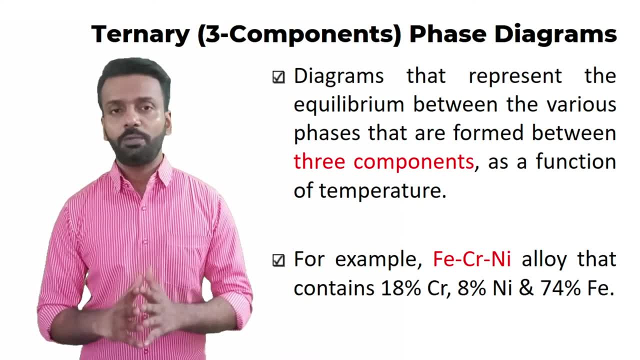 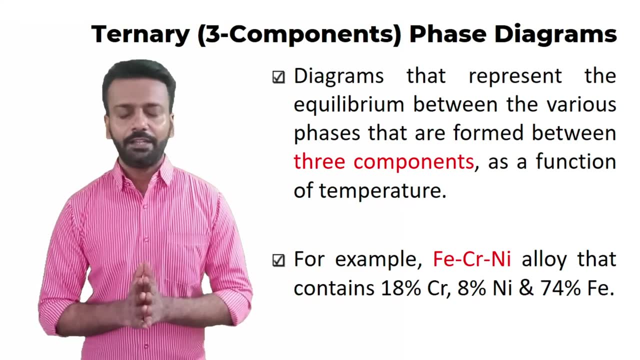 So in ternary phase diagram there are three components which are there and they are plotted against temperature. So as an example, we can see here that iron, chromium and nickel alloy is an example of a ternary phase diagram And we will see in an upcoming slide how we can find out what are the different phases that are existent and how a typical ternary phase diagram looks like. 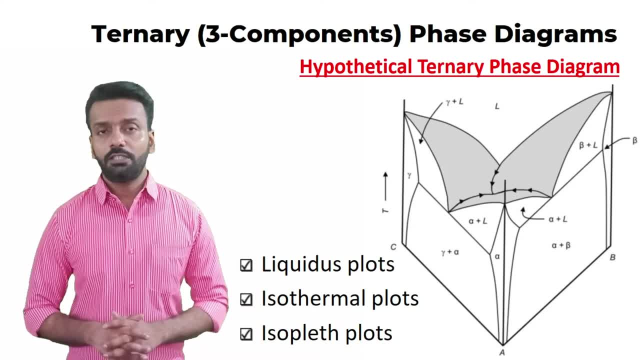 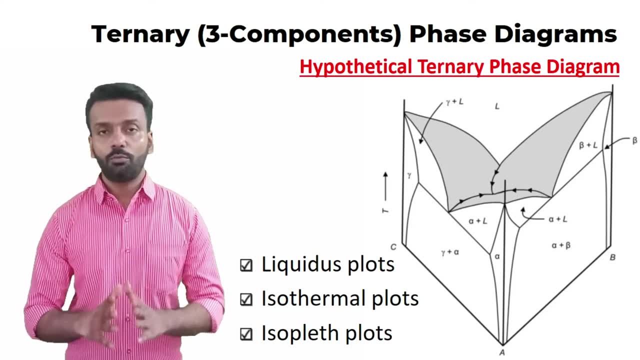 This is an hypothetical ternary phase diagram of three components: A, B and C. So on the x-axis you can see that we have these three components at the corner of this image, And on the y-axis, vertically, we can see temperature. 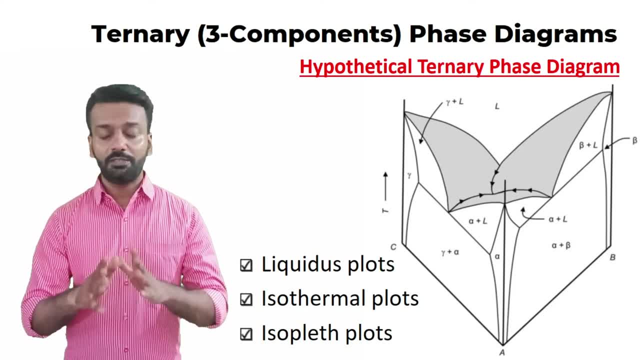 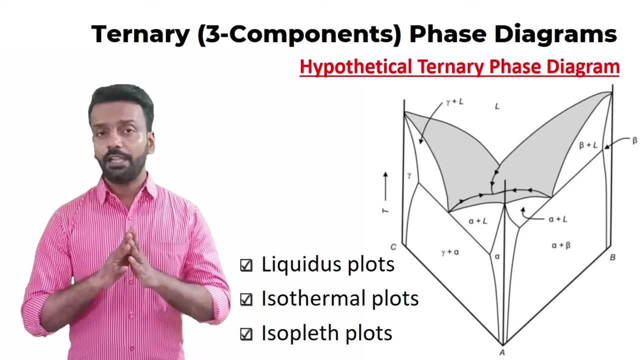 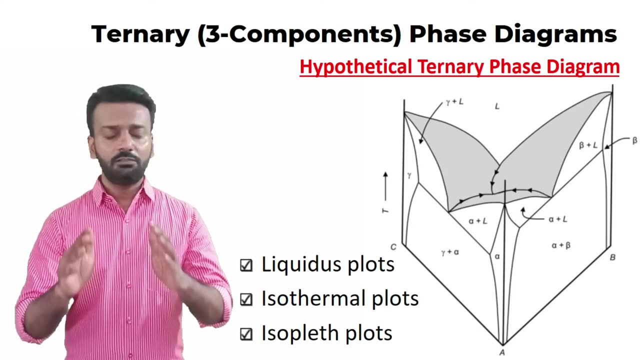 And the dark side of the image or the dark color of the image represent that at this particular time or at this particular point in the ternary phase diagram, the entire phase is liquid And as you are reducing the temperature from that point downwards, the material will change the phase and it will go into a solid phase. 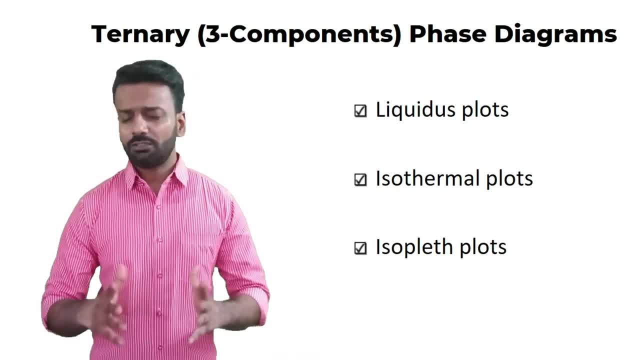 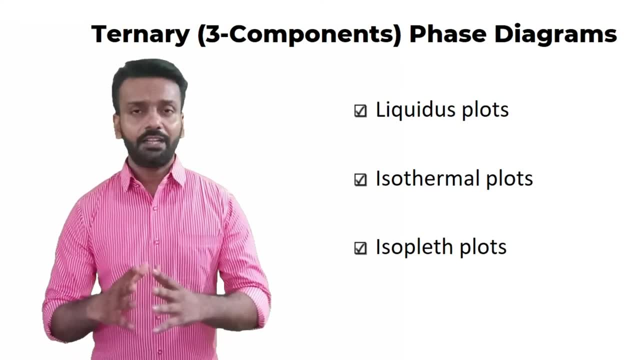 So the earlier image which you saw of the ternary phase diagram was very complicated And it is very difficult for us to read the different phases and to see what phases are existent at a particular point. So for the ease of reading, the ternary phase diagrams are plotted in three different plots. 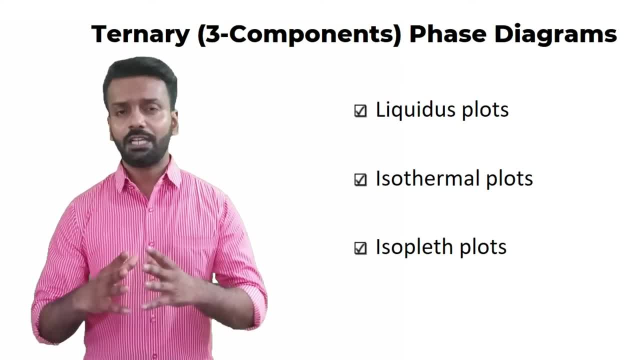 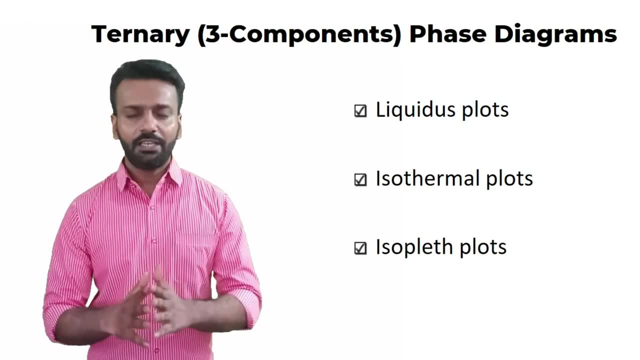 So these plots are liquidus plots, isothermal plots and isoplate plots. So I have decided that I will make a separate video on ternary phase diagram. That is why I will just discuss an example of isothermal plot, and that too, in a very short explanation. 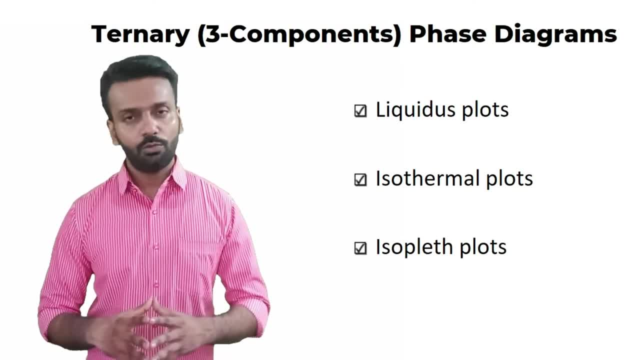 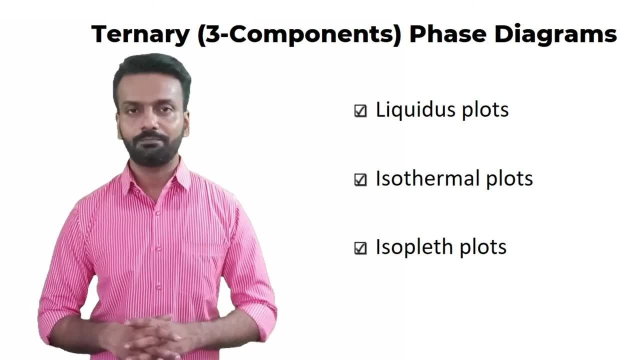 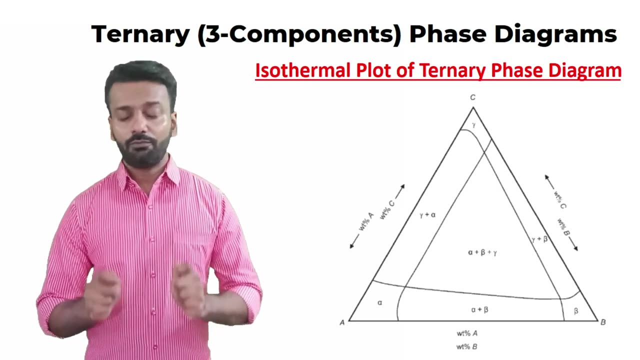 So let us see What are the isothermal plots of a ternary phase diagram looks like and how we can see what are the different phases which are present at a particular point in the ternary phase diagram. So this is an image of a isothermal plot of a ternary phase diagram and this is at one particular temperature. 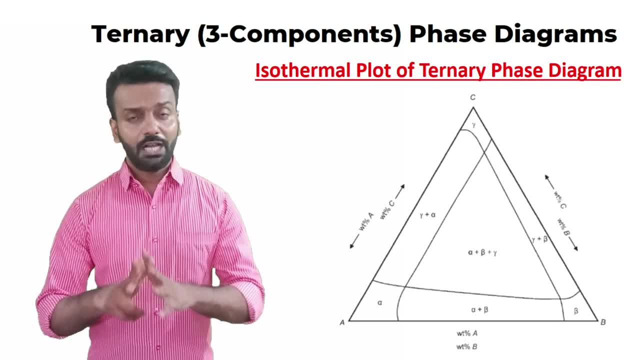 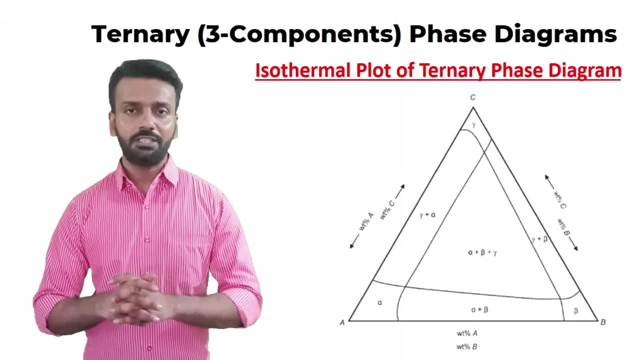 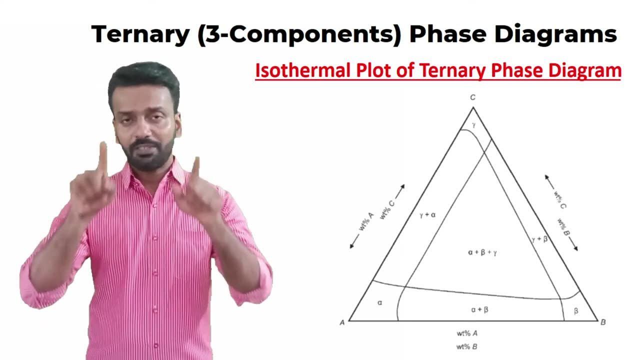 That is why it is called as an isothermal plot. So isothermal plot means it is at a constant temperature. So you can imagine the earlier 3D image of the ternary phase diagram And at one particular temperature you are taking a slice of that particular temperature and then you are representing that in a 2D image or as a two-dimensional image.